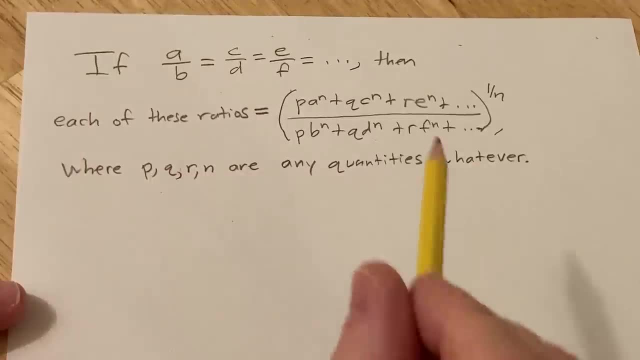 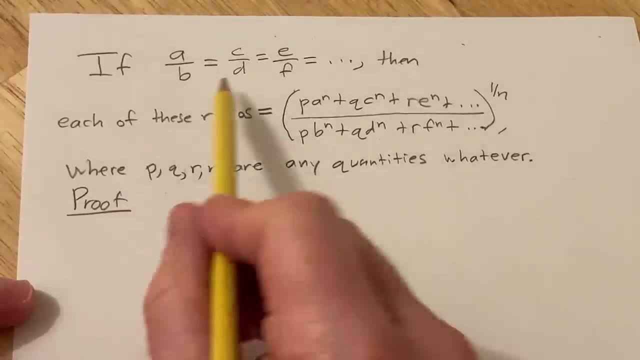 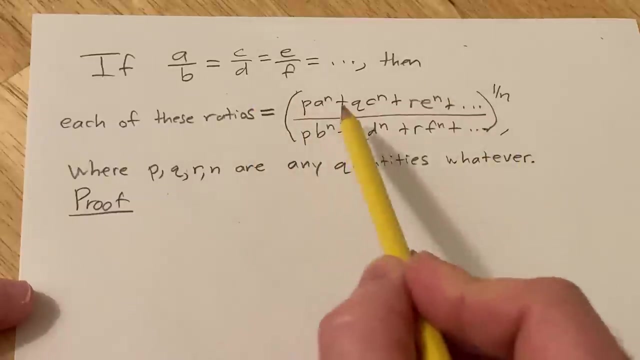 where p, q, r, n are any quantities whatever. So let's go ahead and work through it Proof. So we're going to start by giving this a name, right, because these are all the ratios. So we have to show that all of these are equal to this expression here. So let's give this a name. 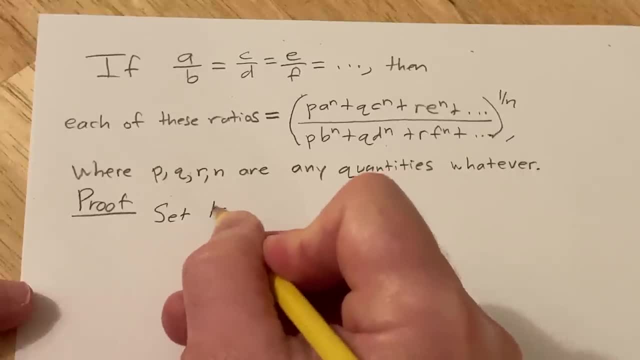 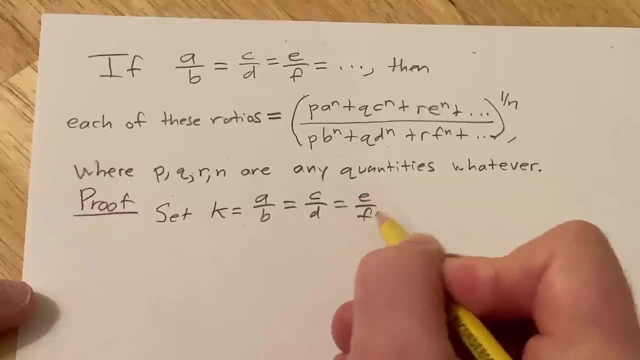 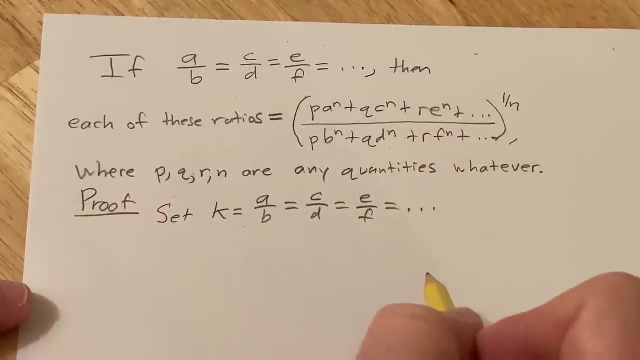 So I'm going to say: set k equal to a over b, which is equal to c over d, which is equal to e over f, etc. right, That's the assumption. So we assume all of these are equal and let's give it a name. And now what you can do is basically I can write each of these: 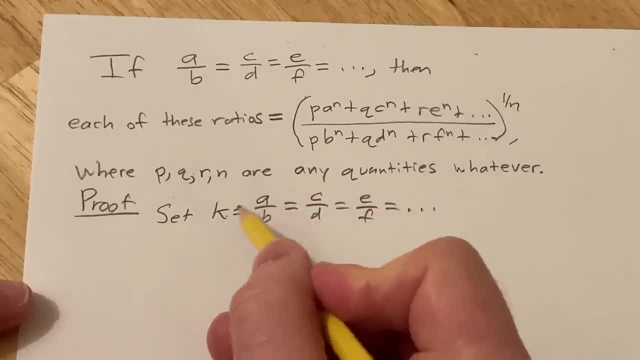 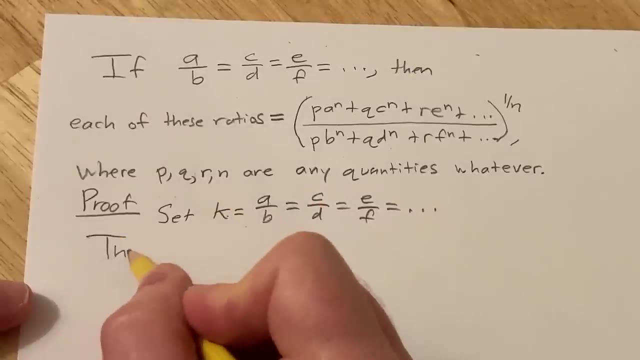 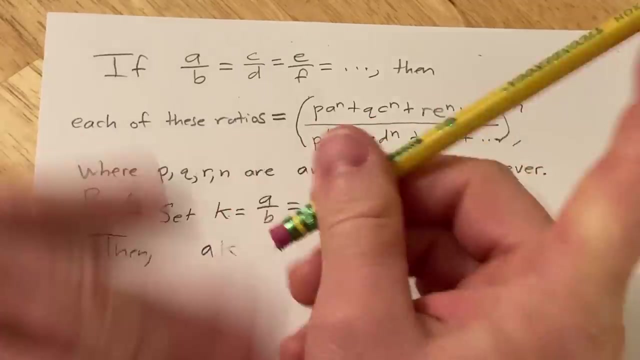 numerators in terms of k. So for example, if I have k equals a over b, I can multiply by b. So then that tells us that a is equal to whoops, a is equal to b times k and then c is equal to d. 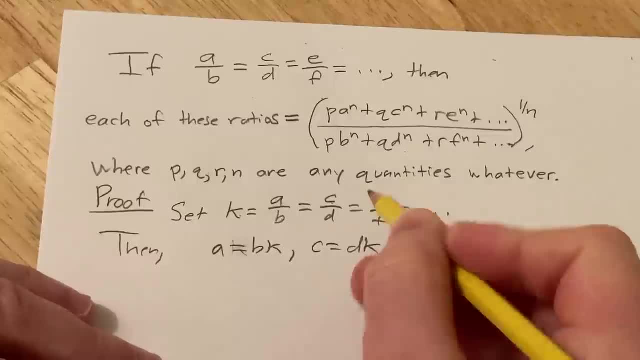 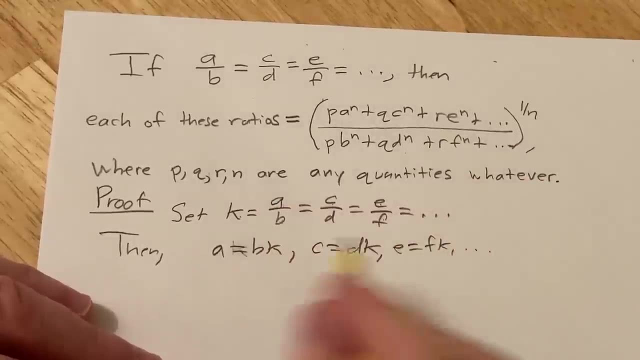 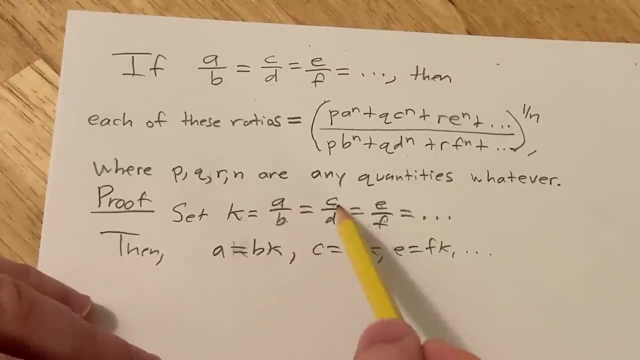 So that tells us that a is equal to d times k, and then e is equal to f times k, etc. right? So again, just multiply by b here. If you have k equals a over b, you multiply by b, so you get a equals bk. If k equals c over d, you multiply by d. you have c equals dk. 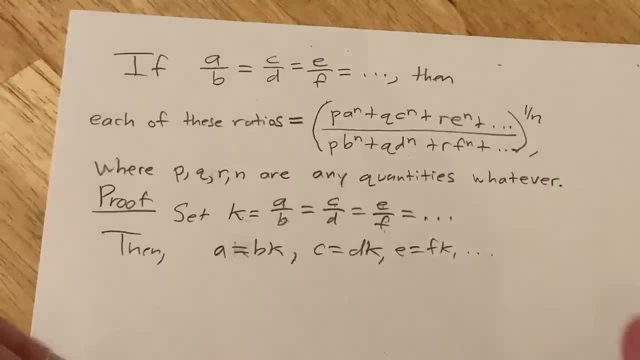 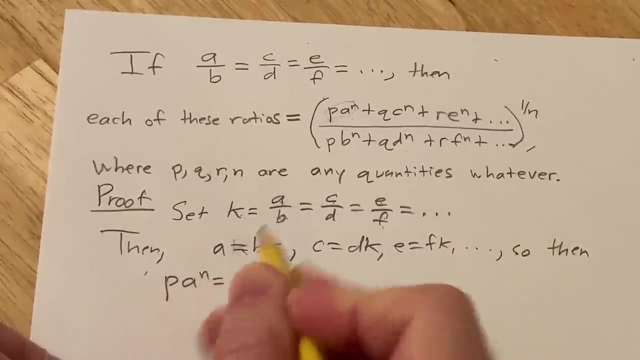 If k equals e over f, multiply by f, you have that All right. so now let's actually work this out. Let's work out what is this numerator here? What is this piece? p a to the the n. So then p a to the n is going to be p, and it's going to be b to the n, k to the n. 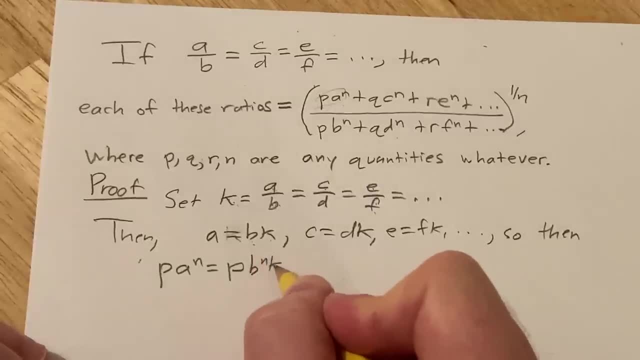 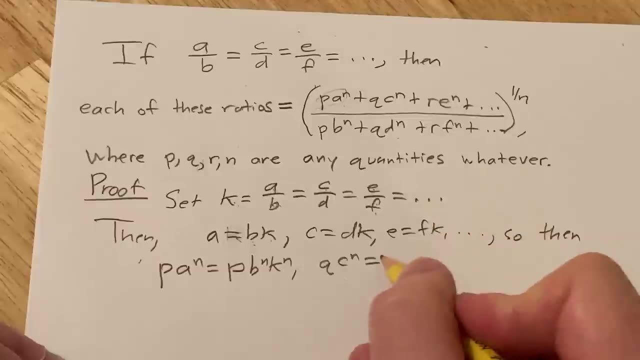 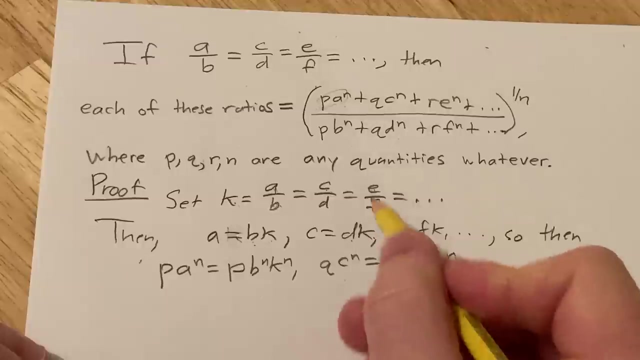 because you're raising it to the nth power. so it'll be b to the n, k to the n And then q c to the n. so q c to the n, it's going to be q d to the n, k to the n And then r e to the n. 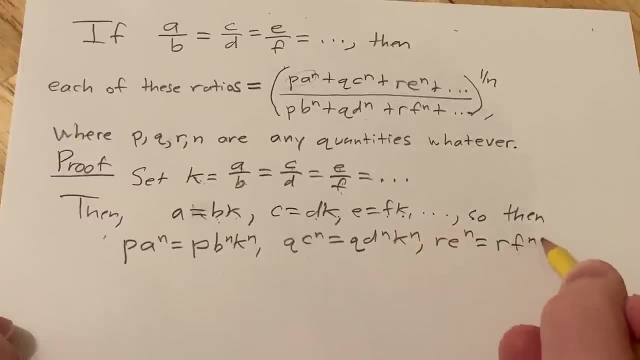 is going to be r, f to the n, k to the n, so f to the n, k to the n, etc. All right, so we've worked out the numerator, at least what's visible here. right, because this goes on. 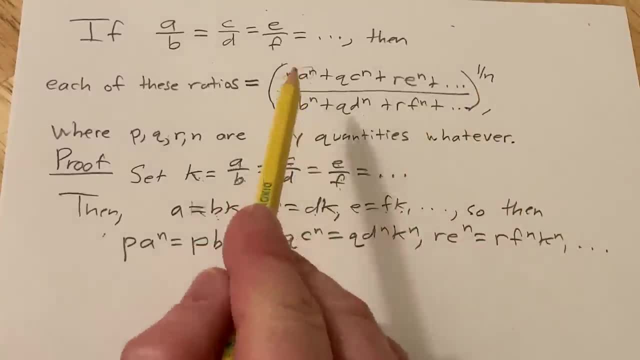 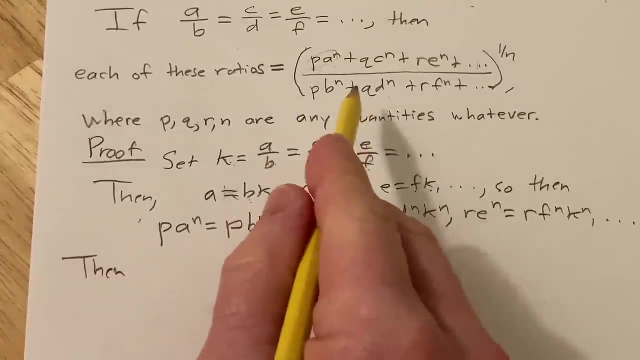 we don't know how far it goes, And so now we're going to write this down. So then, so I'm going to write the whole thing down just as it is, first without the one over n. So p, a to the n plus q, c to the n plus r, e to the n. 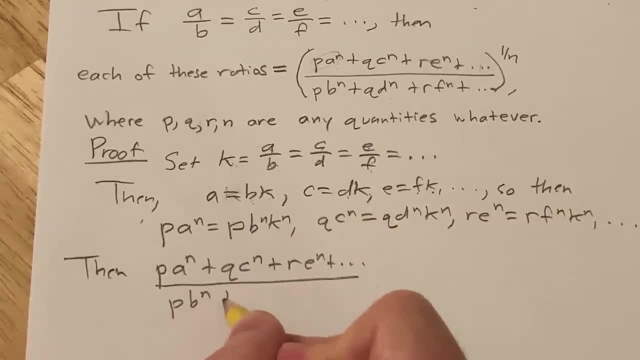 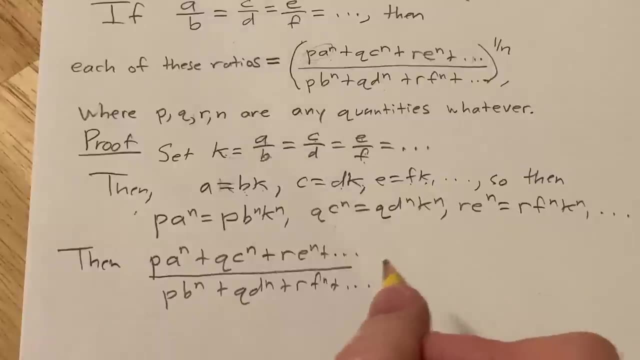 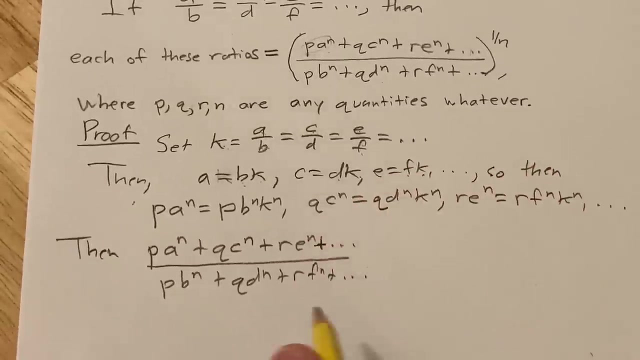 over, and then we have p, p to the n plus q, d to the n plus r, f to the n. By the way, the reason this proof is important is because you can do a lot of other problems using this technique. So that's really the cool thing about it, And we'll talk. 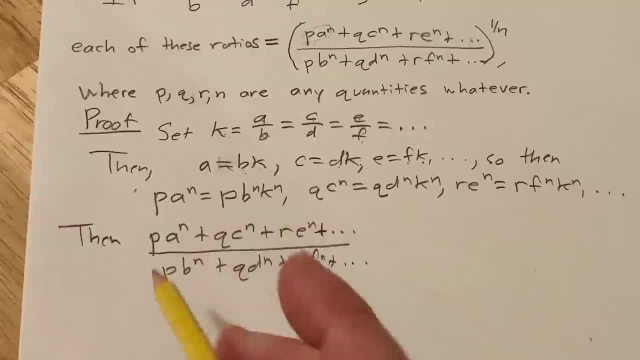 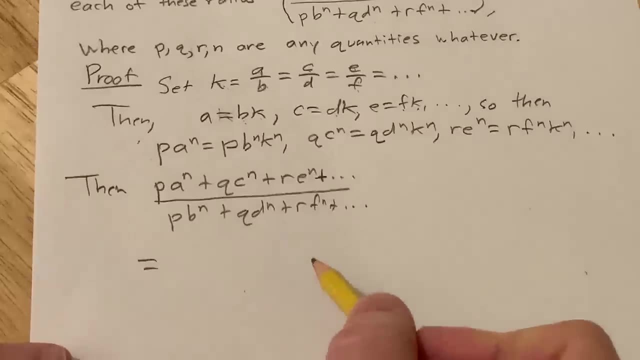 a little bit more about some applications of this once we're done. So. now we can replace what we've worked on here. So this is equal to. so p a to the n is this: so it'll be: p b to the n, k to the n, q c to the n is this: 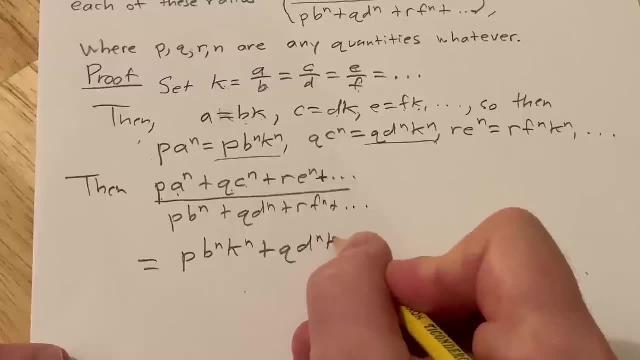 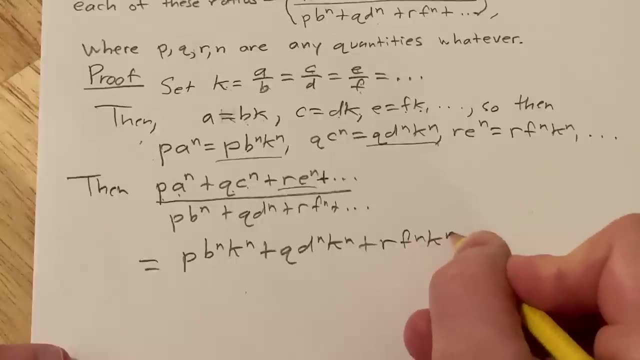 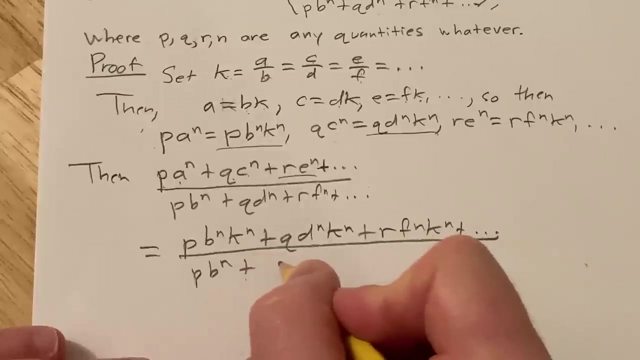 so it's q d to the n, k to the n and then r e to the n. is this so that's r f to the n, k to the n, etc. Then we still have the bottom piece: p b to the n plus q d to the n plus r f to the n. 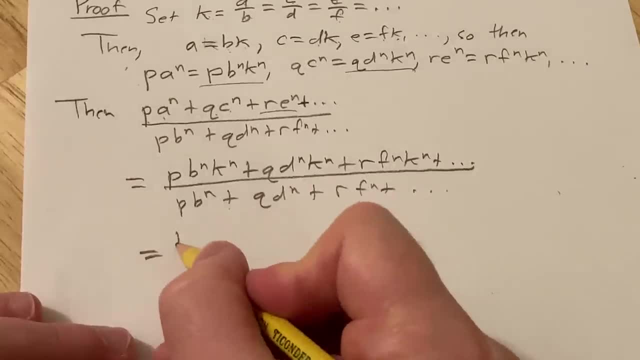 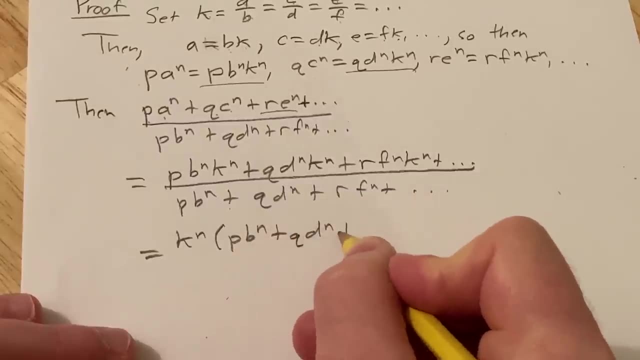 And look at this. you can pull out a k to the n in the numerator, so we have k to the n, we have p, b to the n, plus q, d to the n, plus r, f to the n. There's a lot of variables, right? So it's really easy to. 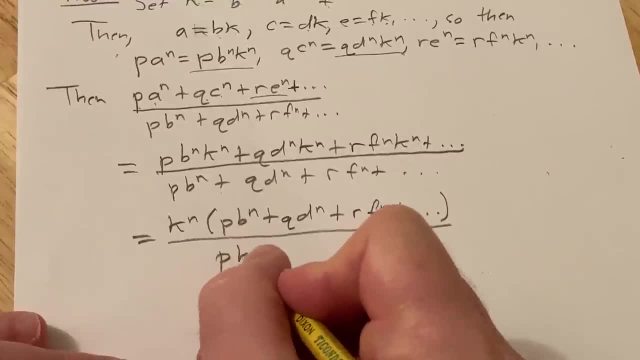 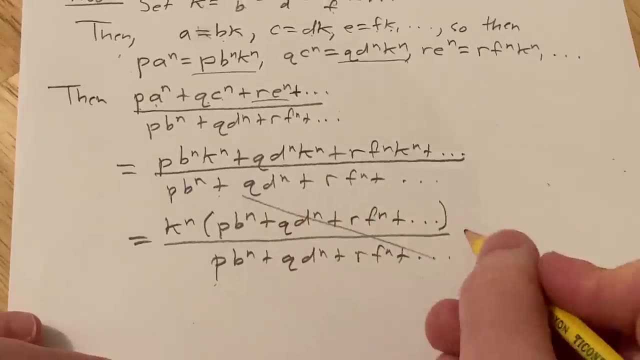 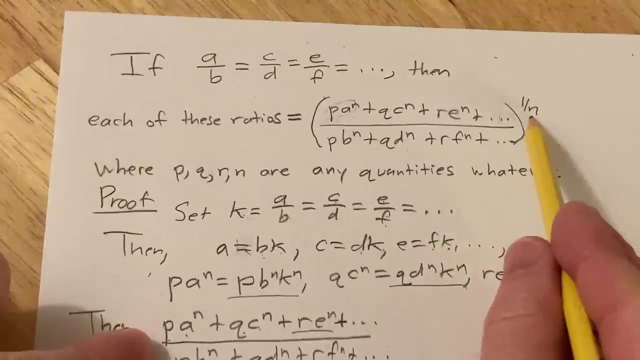 get mixed up, And this is p, b to the n plus q, d to the n plus r, f to the n. These cancel, so this is k to the n. So now we need to take the nth root of this right, Because if you raise this to the 1 over n power, we have to show it's equal to each of. 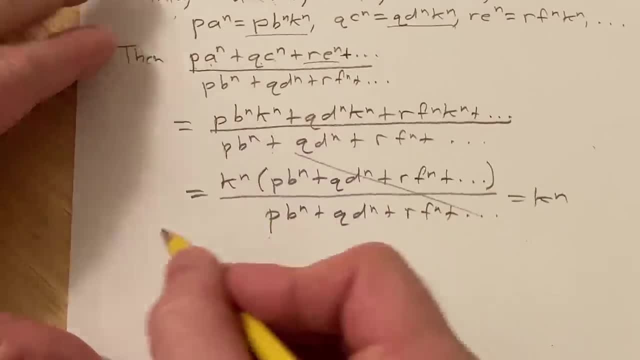 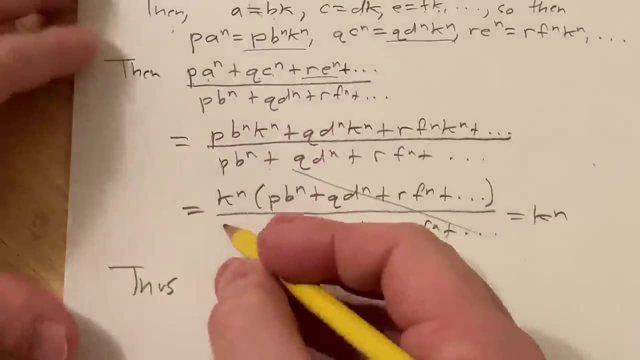 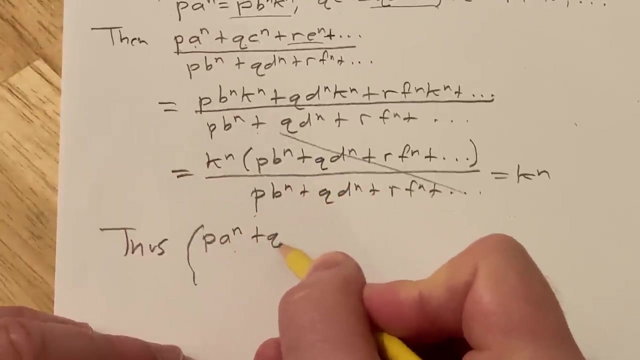 of these ratios. so watch this. I'm going to go ahead and write this down again. So thus our original expression, which was this one to the 1 over nth power. so I'll write it again. so it was P, A to the n plus Q, C to the n plus R, E to the n over, and then 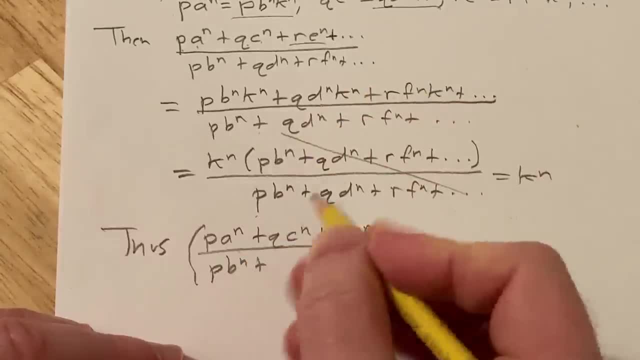 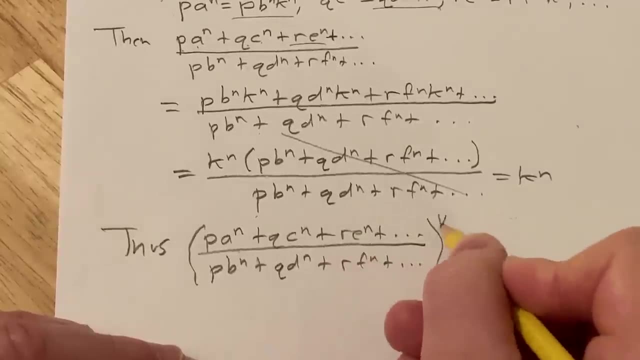 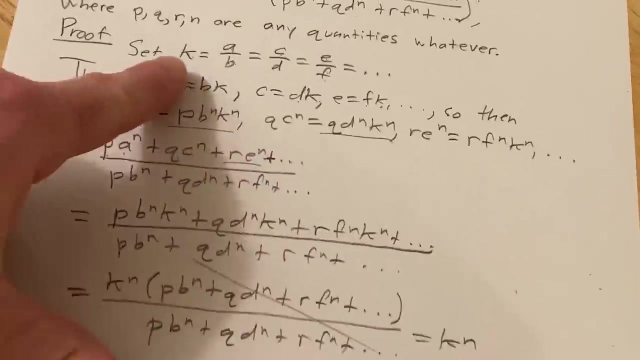 we have the bottom piece here: P B to the n plus Q, D to the n plus R, F to the n to the 1 over n, that's equal to K, to the n to the 1 over n, which is equal to K. but K is equal. 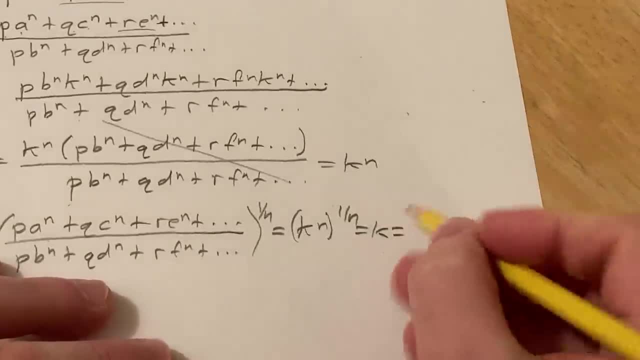 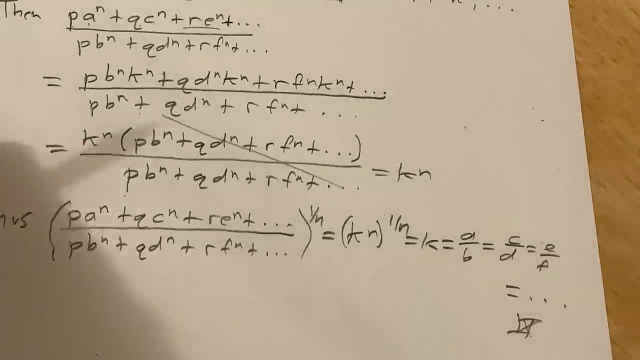 to all of the ratios. we said that at the beginning of the problem. so this is equal to A over B, which is equal to C over D, which is equal to E over F, etc. and that completes the proof. So let me just show you the book really quick, because the book talks about why this is important. 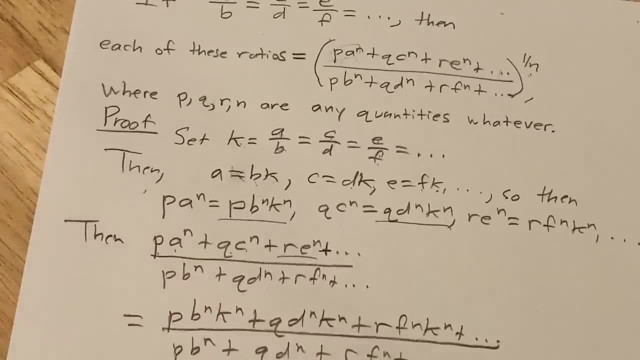 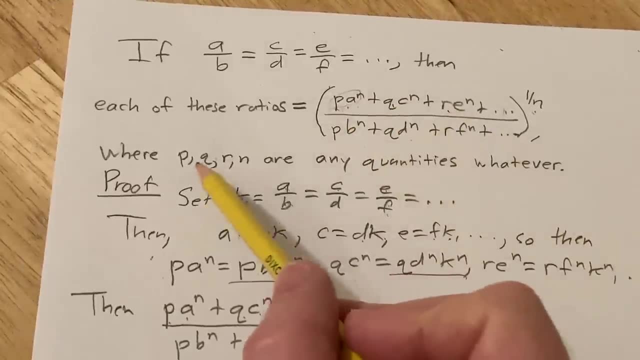 it gives you a specific case of what's happening here. so if you notice, here you have P, A to the n, Q, C to the n, R, E to the n, etc. so if you take, say you take all of these, 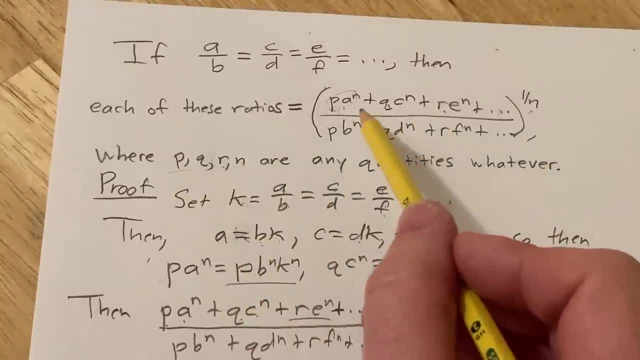 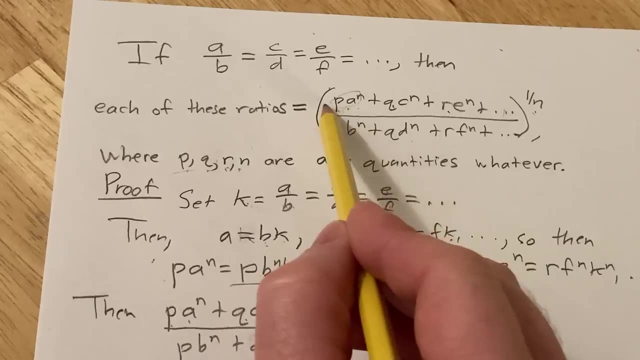 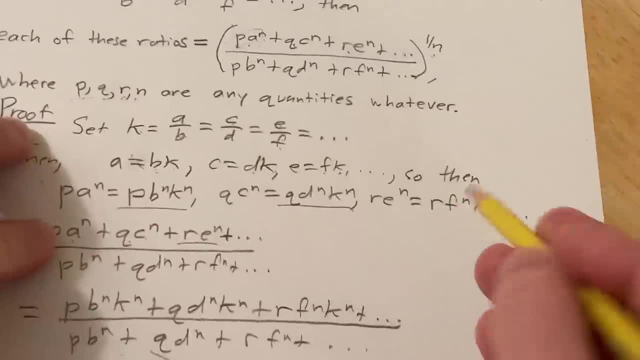 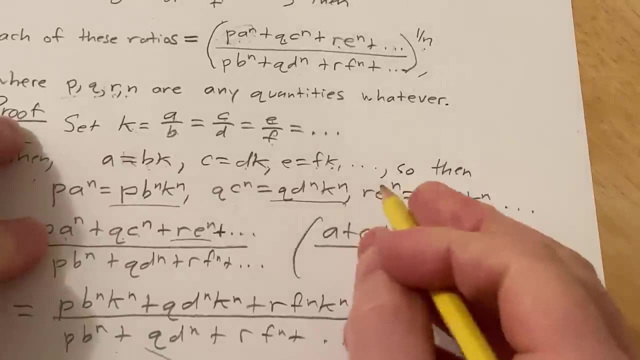 so you would just get A plus 1 over N, right? so you would just get A plus 1 over N, right? so you would get A plus C plus E. so you would get A plus C plus E over, and then on the bottom, 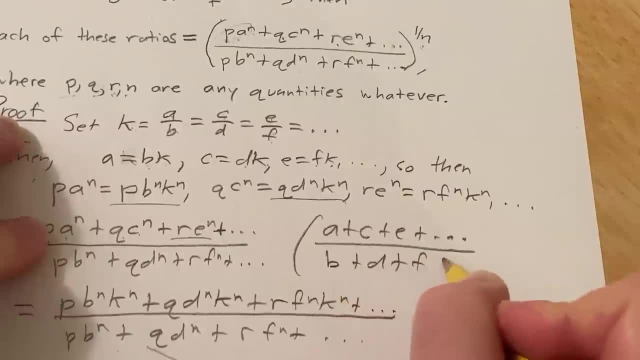 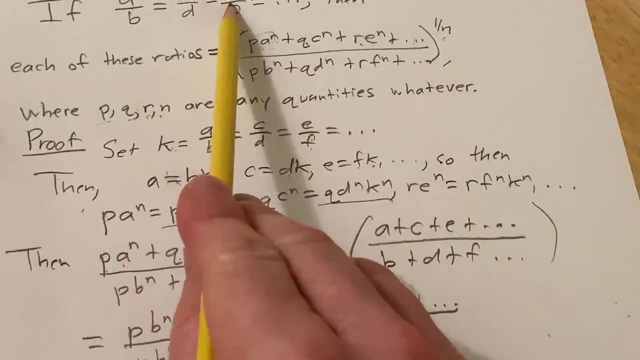 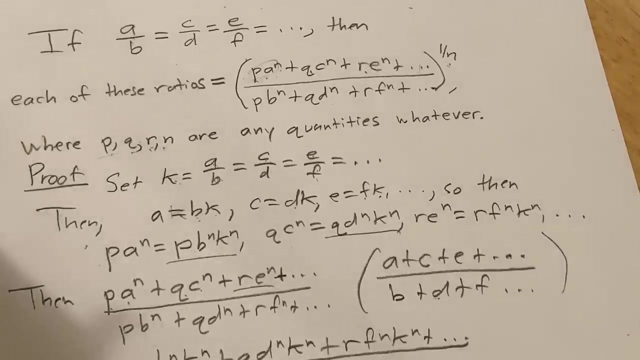 you would get B plus D plus F, right? so basically, when these ratios are equal, the ratio of the sum of the numerators to the sum of the denominators is also equal. that's what this is saying, right, and the book talks about that. let me show you it says it, let me. 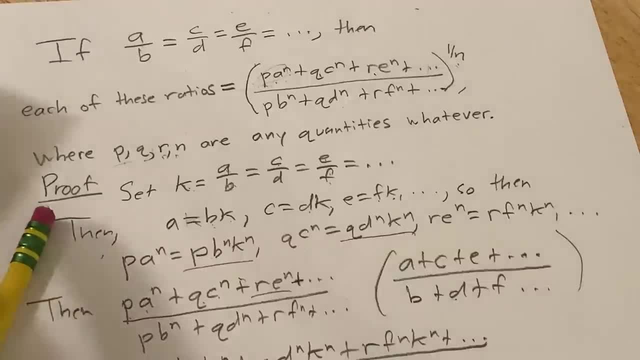 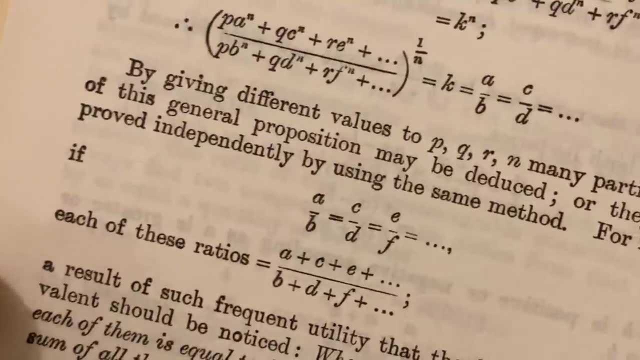 just find it for you. It's pretty cool. I was just sitting here working and I thought, hey, I should just show you this proof. so it talks about it here. it says: by giving different values to P, Q and R in many particular cases of the general proposition may be deduced or: 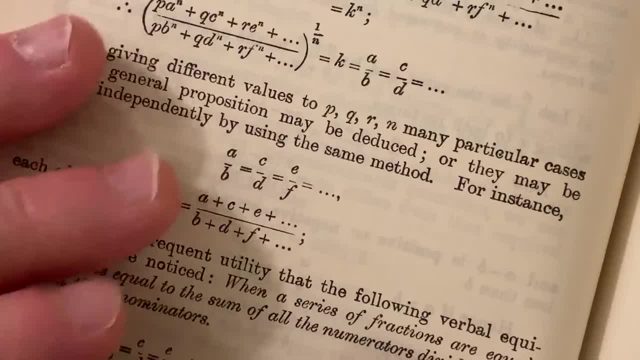 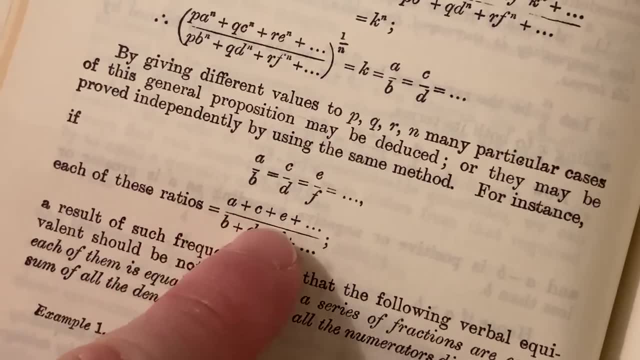 they may be proved independently by using the same method, right? so the method of this proof will allow you to do other problems. for instance, if the ratios are the same, then each of the ratios is the sum of the numerators to the sum of the denominators. 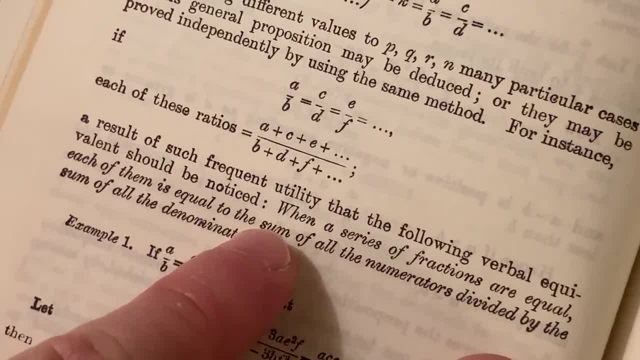 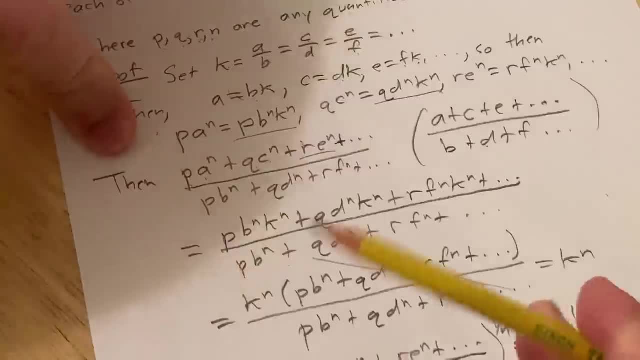 right, so it says it here: When a series of fractions are equal, each of them is equal to the sum of all the numerators divided by the sum of all the denominators. so kind of an interesting thing, right. so if you had, just as another concrete example, say you had, you know, it's maybe simple algebra.